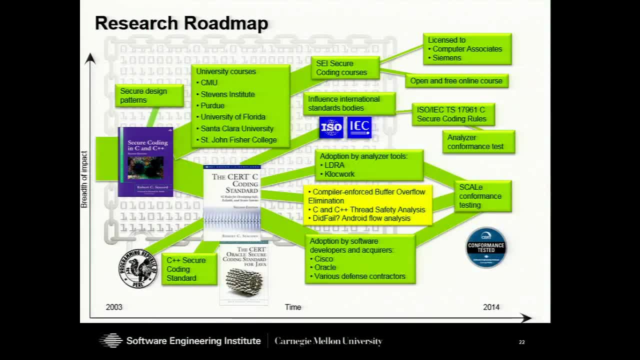 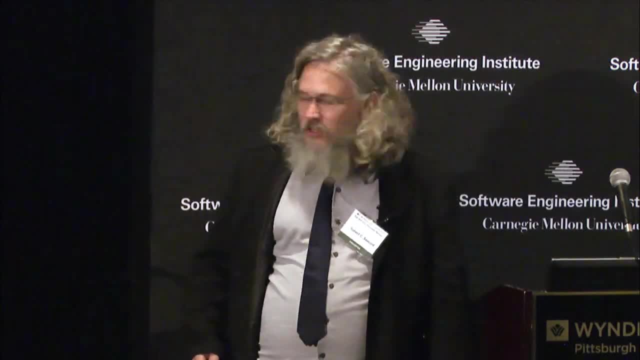 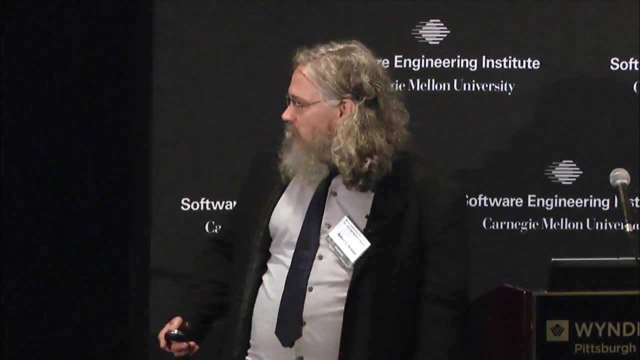 a standards meeting in Berlin in 2006 and suggested CERT develop a secure coding standard for C, And I thought that was just a lovely idea. so we- you know a mere- well, you know- two additions and ten years later, we've made quite an investment impact in that area, And this is branched. 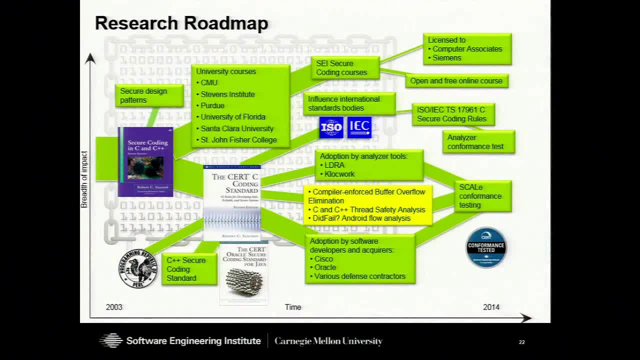 off into a bunch of things. You know, we now have pretty wide adoption of these coding standards by companies such as Cisco and Oracle. A number of defense contractors have also adopted these, But they've done that under NDA, so I can't tell you who they are. They seem to feel that. 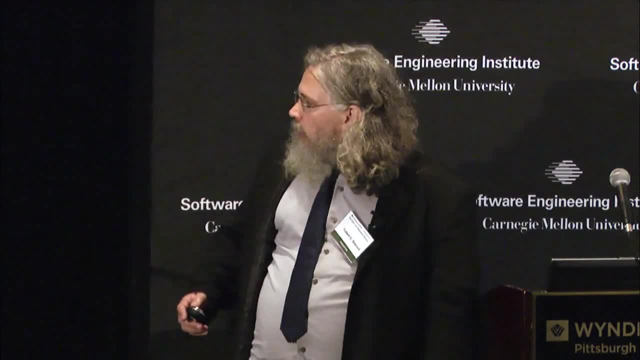 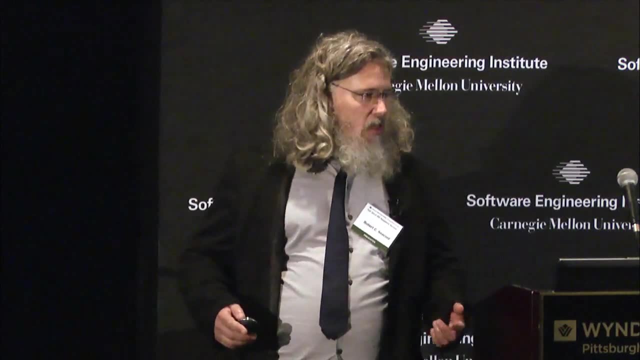 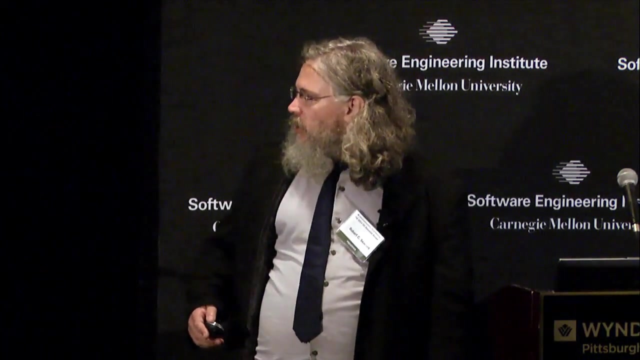 gives them a competitive advantage, And so this work has created a sort of a- well, our scale analysis, which is a collection of static analysis tools that we use to analyze code to see if it conforms to one or more of the coding standards, And a lot of the research. 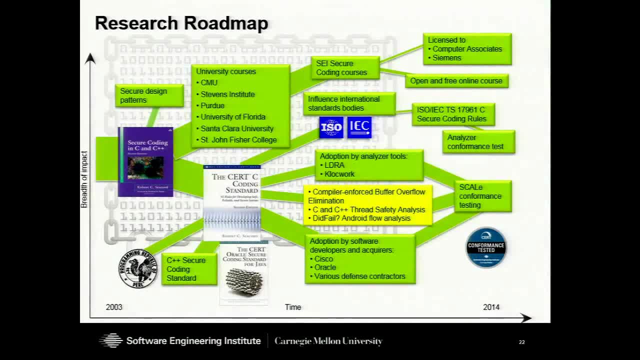 work I'm going to talk about today is in that yellow box. These are all sort of capabilities that we've tried to develop to enhance our ability to analyze code for conformance with our coding standards. So one of these projects that's been ongoing for several years is our compiler-enforced 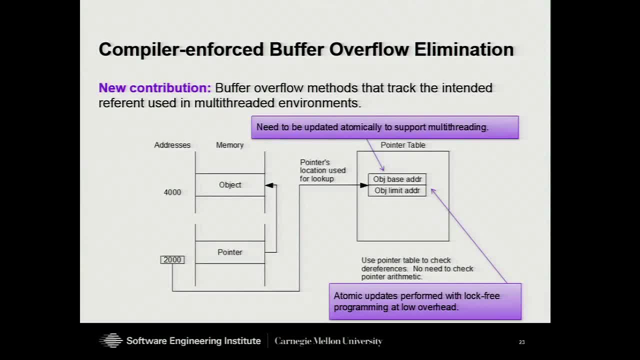 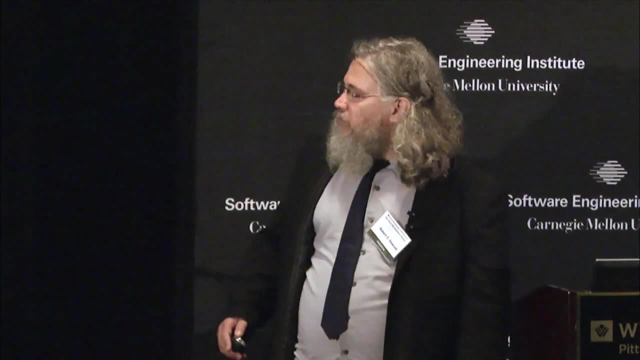 buffer overflow elimination project. This is led by David Keaton. He's the current convener of the WG14C Standards Committee and he's on a number of people's top ten list of parallel computing experts on the planet. So he's- he's a- he's sort of a bright guy. 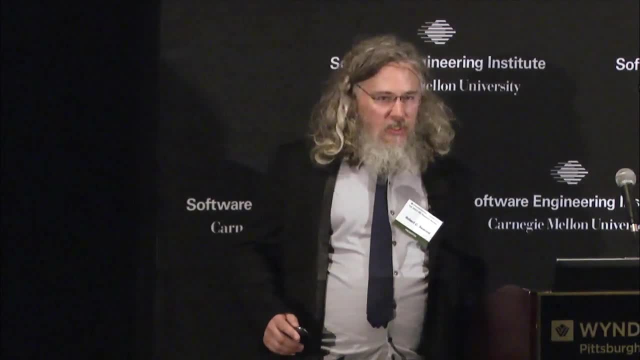 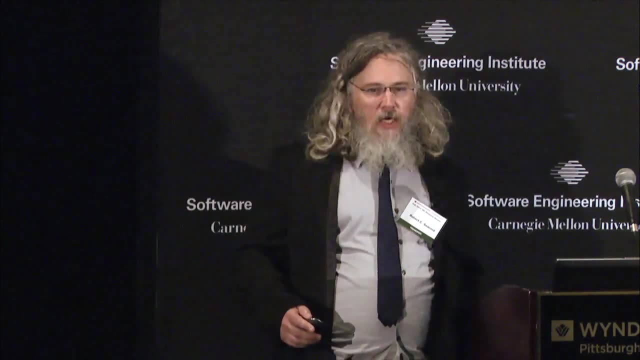 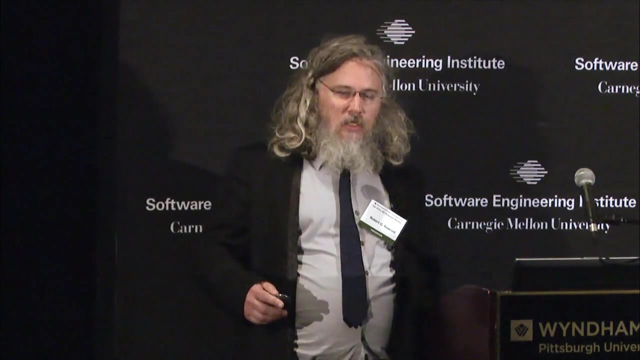 And so he had two major contributions in this work. So one was to to do some optimizations of the Clang compiler to improve the performance of buffer buffer overflow elimination, basically by hoisting checks outside of loops where they will only be performed once instead of. 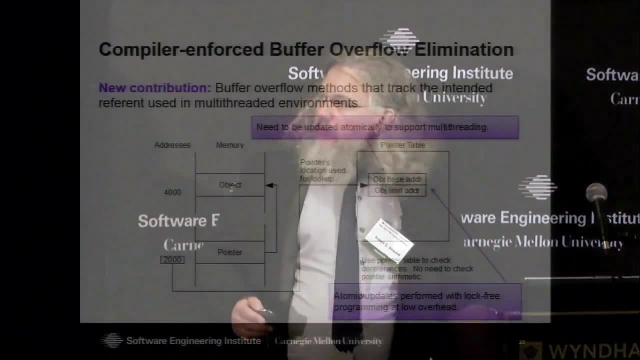 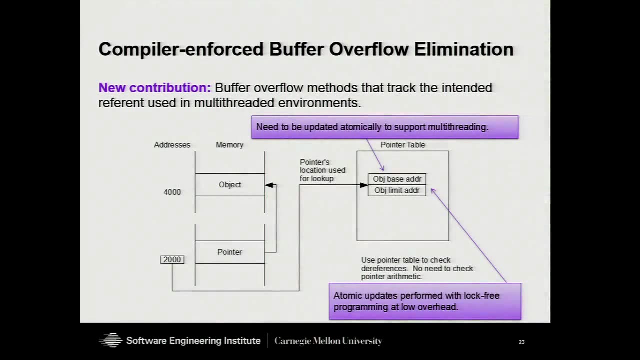 being performed on each iteration. And the second contribution is to expand this work to work with multi-threaded applications, because both C and C++ have had new standards in the last few years where they've basically introduced concurrency into the language, And you know. 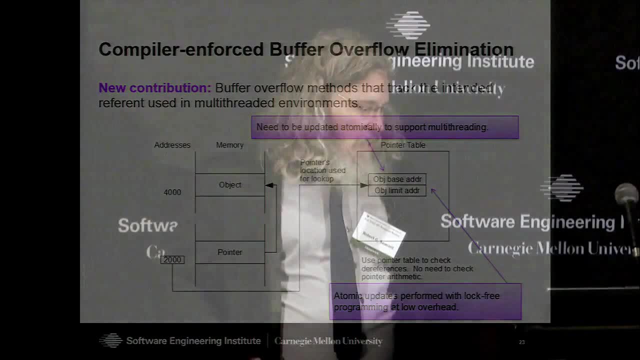 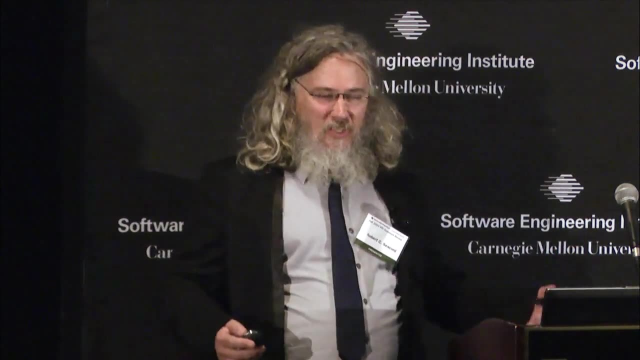 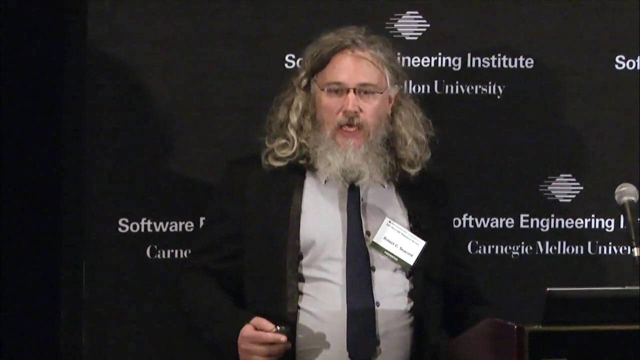 everyone's well aware that this is kind of an important new. you know, I mean, for 30 years people have been saying that. you know, concurrency is eminent, parallelism is eminent. I'm starting to believe it, You know, and, and, and certainly. we're seeing the reaction. 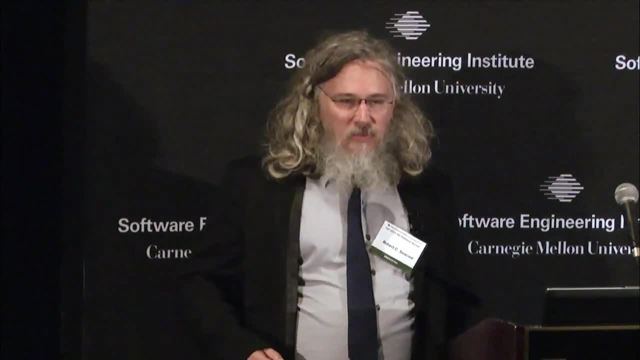 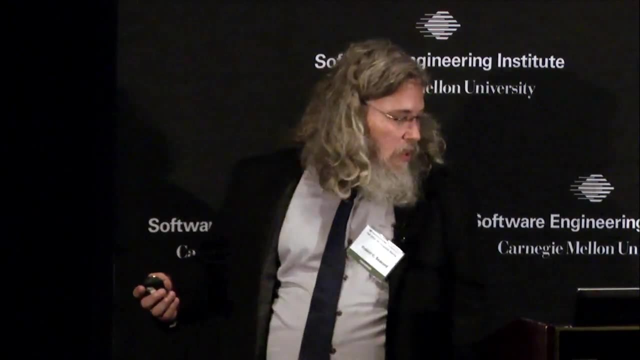 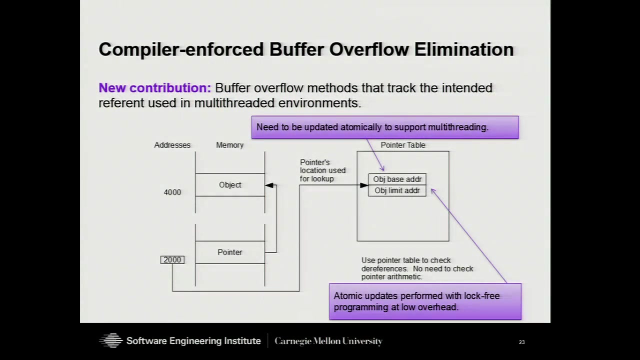 from the language committees. They believe it and you know the entails and everyone else believes it. So part of this work was to basically to use these, these object tables, in order to keep track of the base pointer and the bounds of all the objects, to ensure that each, each, 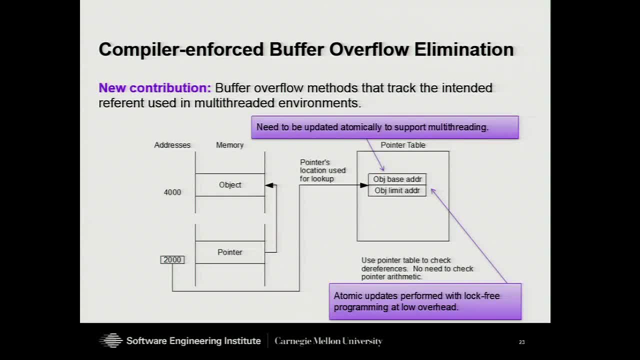 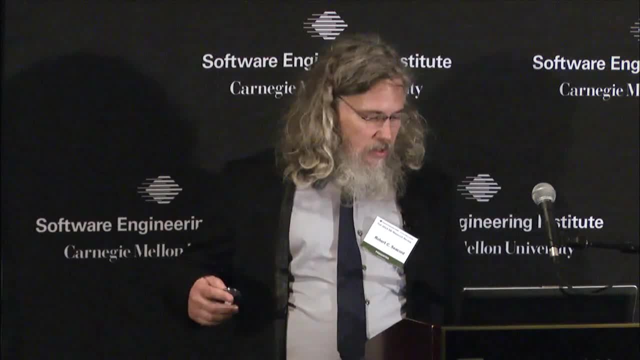 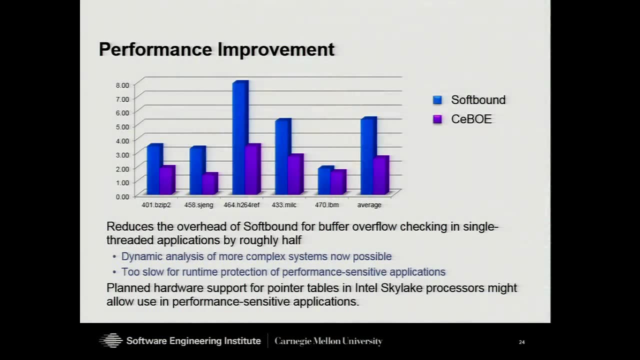 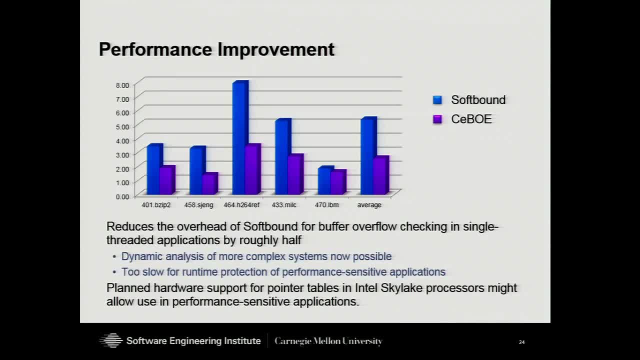 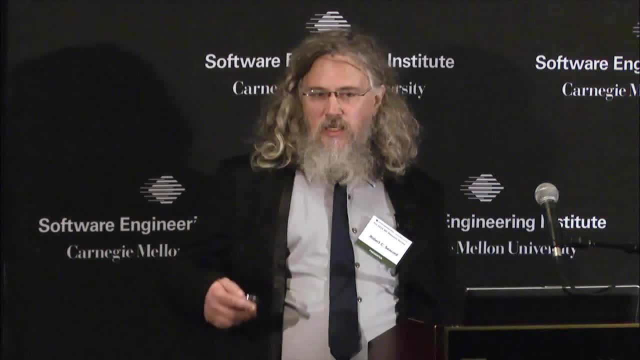 data sets. you can do a lot of trials and шawls before you think about how many you ever had in mind, And that was now what we've been doing. actually L length and л over length And um to what? do you think this is a long term blessing to the answer as to if we could. with a 5% overhead or greater, they sort of laugh you out of the building. So they're very sensitive to performance, And when security and performance go up against each other, security always loses. It's kind of sad, but true. 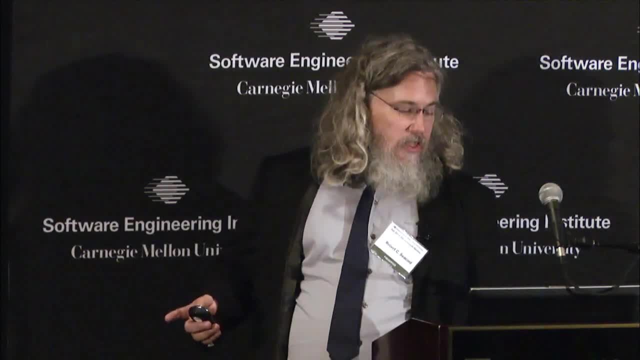 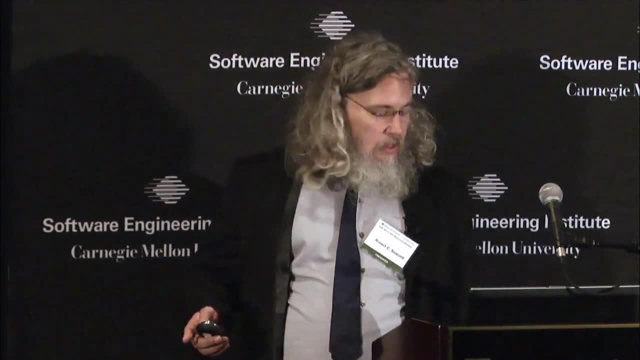 But one of the things that we're looking is that there is going to be planned hardware support for pointer tables in the Intel Skylake processors And once that hardware support is there, this solution might actually become quite viable for a wide range of applications. 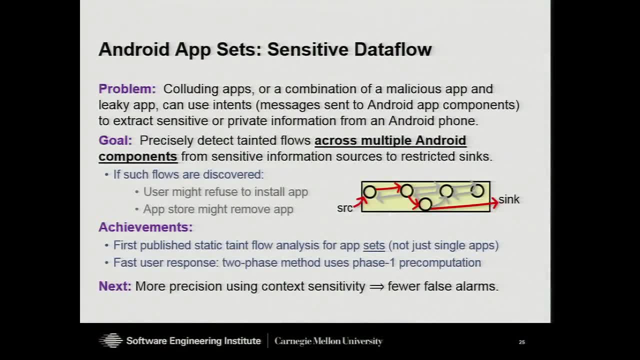 Another project that's been managed by our two PhDs, Laurie Flynn and Will Kleber, along with the ECE staff, is this data flow for Android app sets, And so the problem here is that you can have a number of apps on your Android phone. 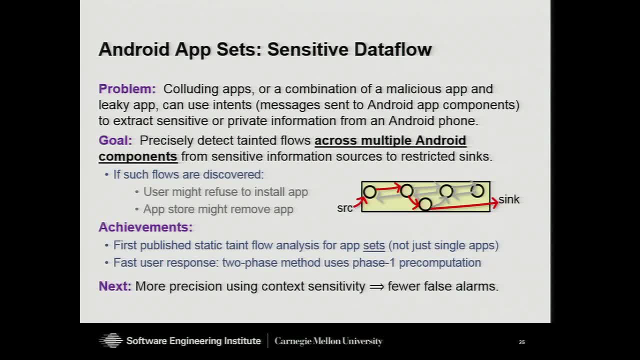 which appear to be quite secure, but in collusion with another app, they can leak sensitive data from your phone, and that's largely undetected, particularly if you're analyzing each app in isolation. So there's this problem with what's called intents. 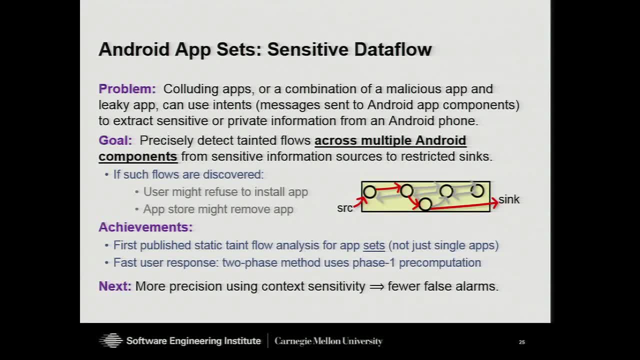 which are basically messages passed between these components, and existing analysis fails to detect these data flows. So our research team set off to precisely detect these tainted flows across these multiple components and allow the user to refuse to install the app or for the app store to maybe not install it. 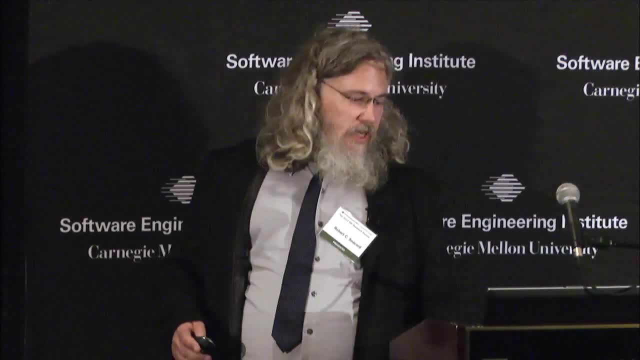 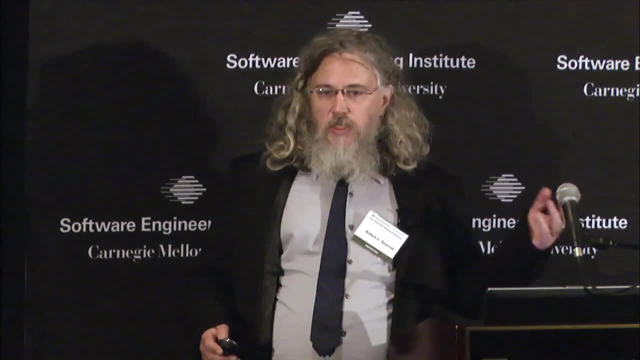 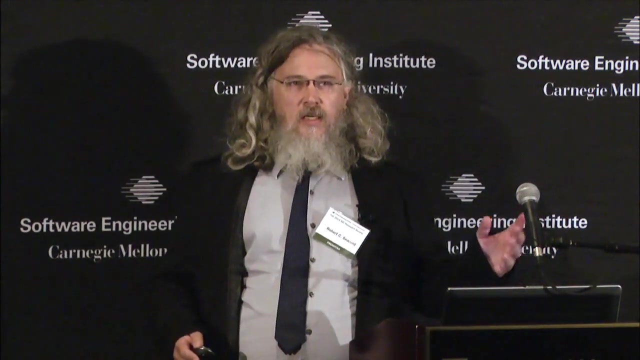 So this was the first published static taint flow analysis for collections of apps And they use basically a two-phase method Once, where they initially analyze the app, say, before it goes into the app store, so they can do stuff which is slow. 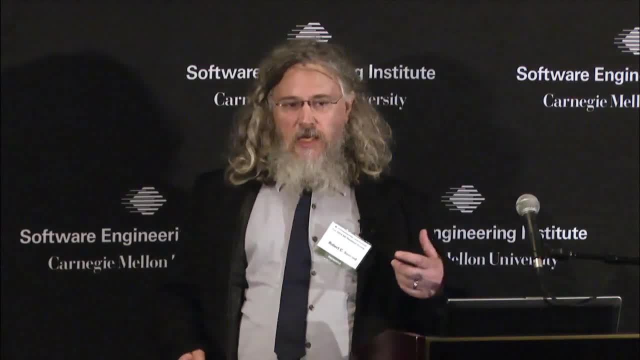 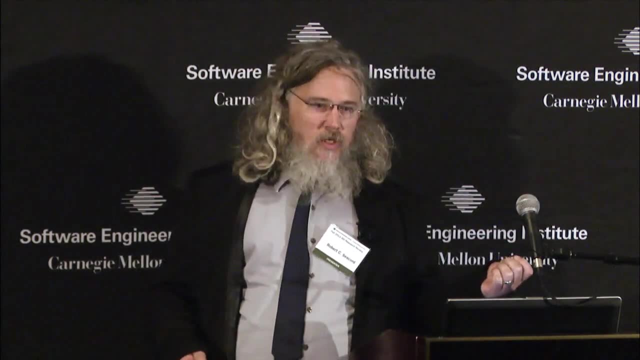 Right, it's not time critical, And then when you go to install an app on your phone, it will then use this information to look at the collection of apps that you're now going to have installed and make sure there are no sensitive flows between that particular collection. 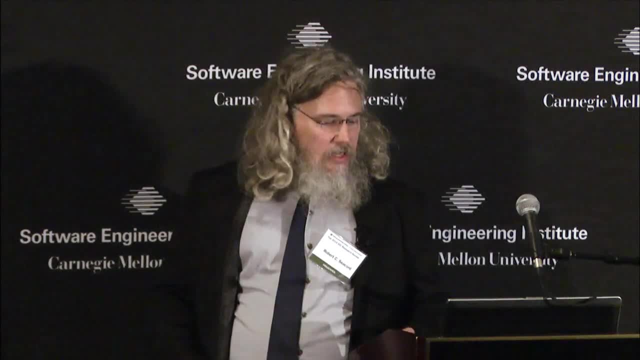 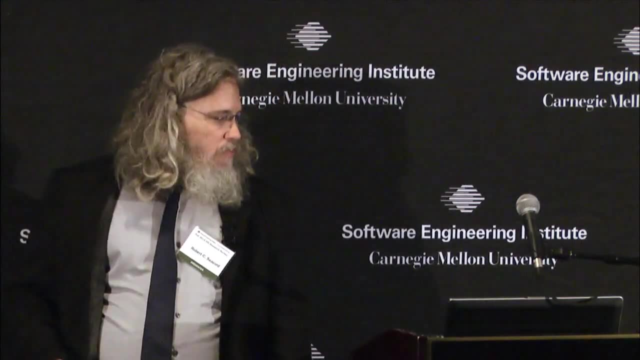 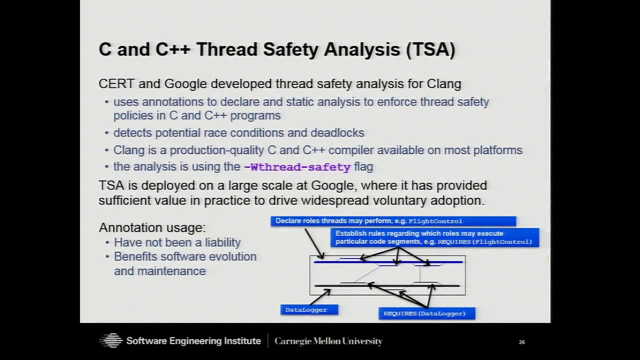 The next steps in this research is to add more precision with contact sensitivity and consequently have fewer false alarms, fewer false positives. The third project I'm going to talk about is our CNC++ Thread Safety Analysis. So this was a project that we collaborated with, with 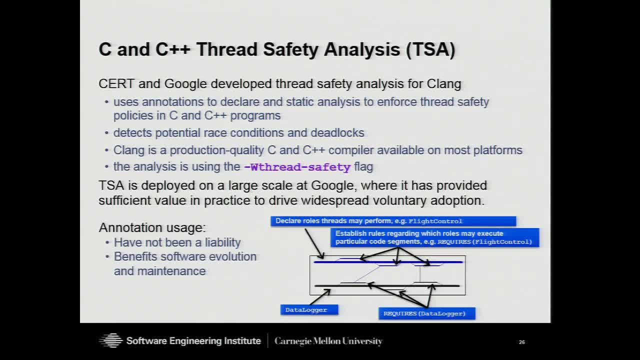 Google. You know, it would have been great if a lot of that collaboration was then giving us bundles of bundles of the money they have, but we got the next best thing, which is we collaboratively developed Thread Safety Analysis for C and C++ programs, using annotations that originated in. 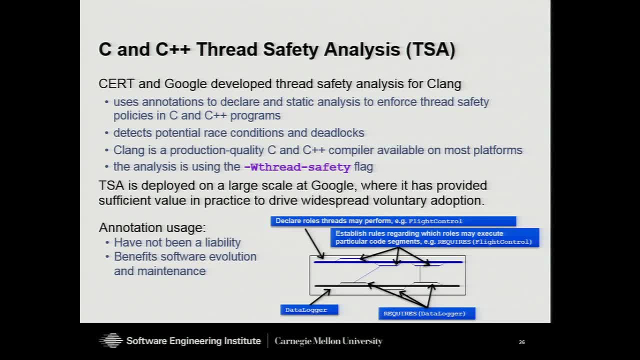 Bill Shurless's fluid lab here at CMU, And so this allows potential race conditions and deadlocks to be detected. This has been implemented in Clang, which is a production quality compiler available for most platforms, and you can basically download and use this at your own organization today. 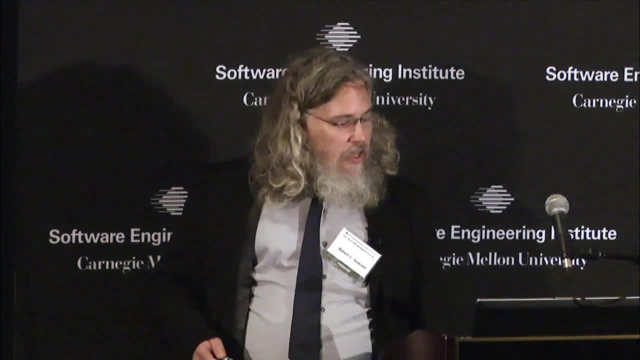 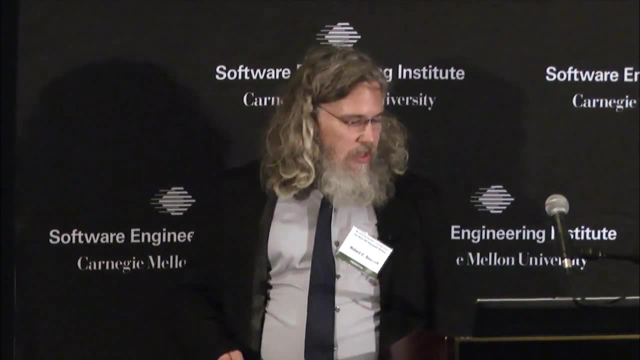 So the Thread Safety Analysis has been deployed on a large scale at Google. It's voluntary but it's been widely picked up, so people see the value of using it and it's being used to develop applications that are used by- you know, probably a billion people. 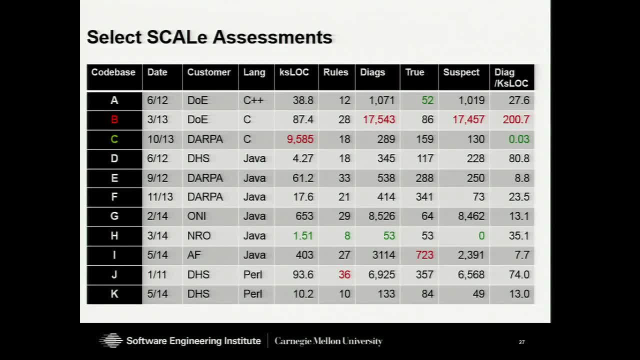 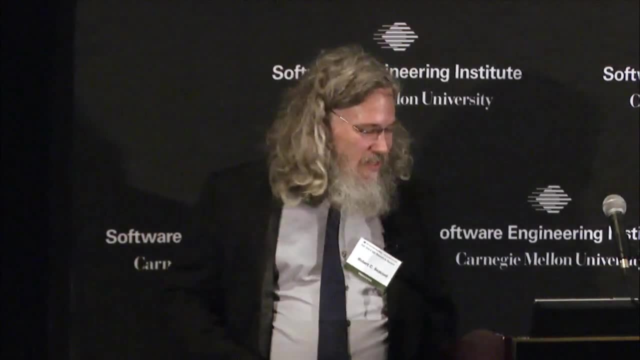 So here's a chart of some of the scale assessments that we've performed over the past couple years. It's an interesting chart and a lot of people sort of find their organizations in this chart and start asking me questions, but I've mostly sort of obscured the specific groups which have developed. 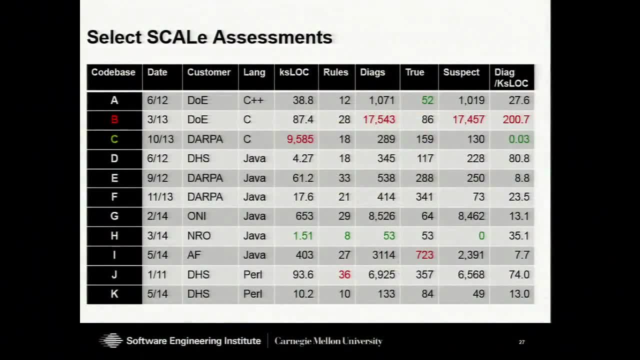 systems. so it's fairly anonymous. what I've done: in each column I've marked kind of the the lowest value, or it's kind of the worst value in red and the best value in green, and what I want to do is call your attention to the B and C. 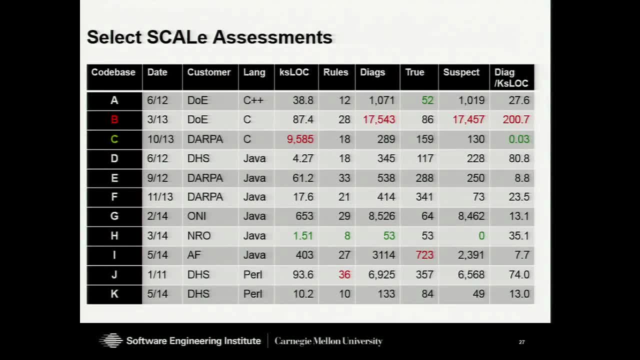 rows. so these are interesting because they are both systems that were developed by commercial software vendors and they were both written in C, and the C row, you see, has the highest quality, the the least number of secure coding violations per thousand lines of significant code of any system. we looked at point zero. 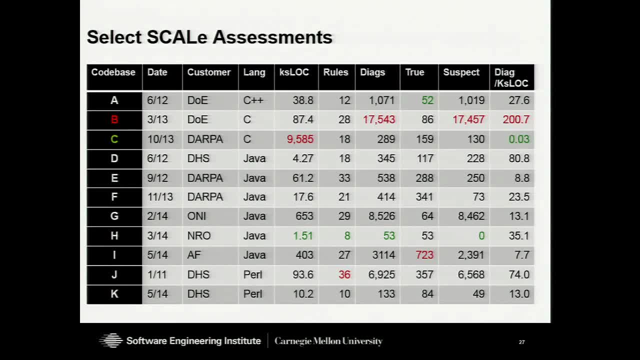 three and the row above it, and it's actually one of the. it's actually the largest system. we looked at the row above it. B is another commercial vendor, also written C, and they have absolutely the worst quality that we've seen: the most defects per thousand lines of significant code. so so what's sort of. 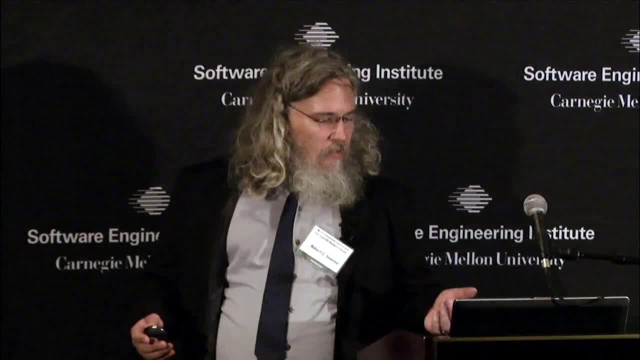 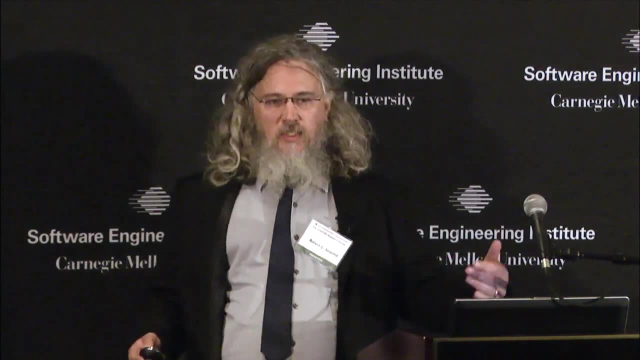 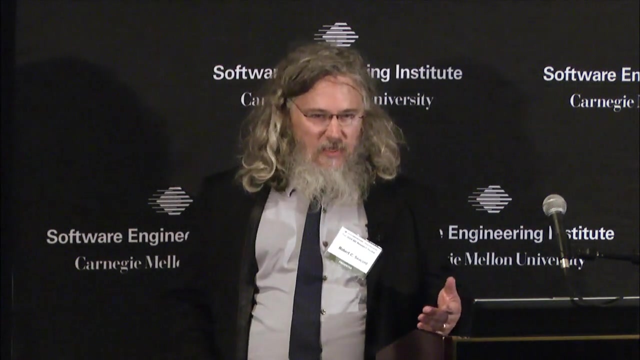 interested in that. there, I think, is that you know, although both these systems are developed in C language and they're both developed by industry, one is the worst and one's the best, and what that sort of gets to is that the real differentiator here is sort of the quality of the developers and and their expertise in in secure 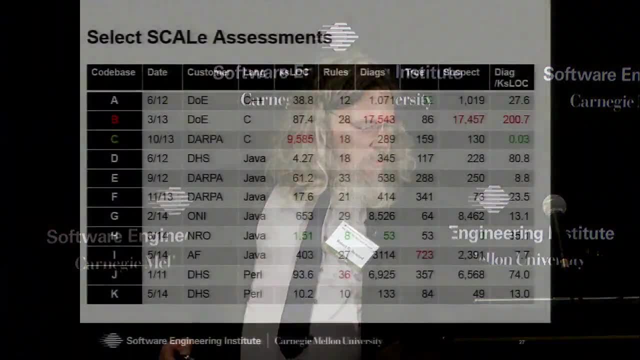 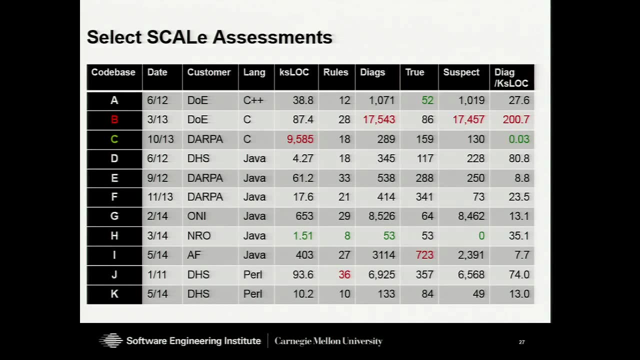 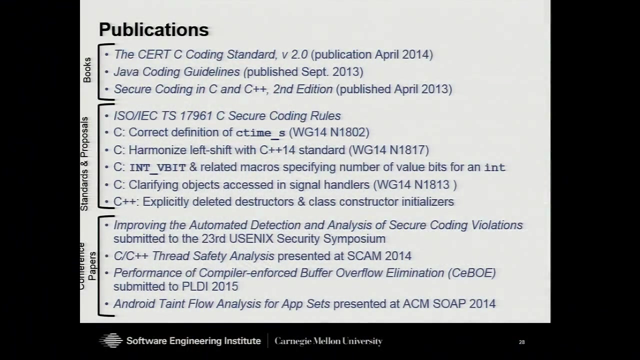 coding, and so I you know. so the good system. I'll go ahead and tell you that's actually the Android kernel developed by Google and deployed by DARPA transfer and the very horrible application. I will tell you who wrote that, because that's kind of embarrassing. so here's just a list of publications that we've had. we 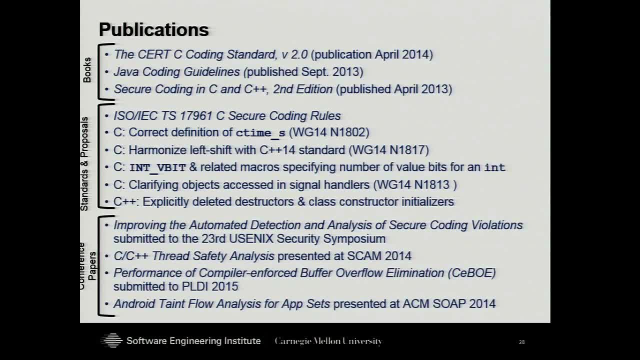 kind of have a slow year for books. I think we only wrote one. my publishers a little bit angry about that. but I'm promising to get back on track and one of the more significant accomplishments here is the 1726 technical specification that we published through the I would ход, I see.